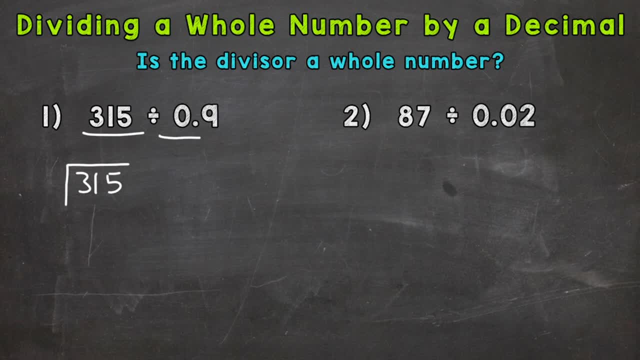 and it goes underneath the division bar and we're dividing by 9 tenths. So that goes on the outside. that's our divisor. So when it comes to division problems that involve decimals, we have that problem set up. but we need to ask ourselves a very important question before we can go through. 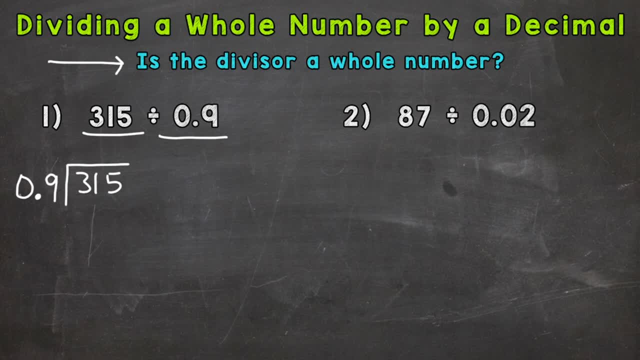 the division process, and it's at the top of your screen. Is the divisor a whole number? And in this case the divisor- the outside number, 9 tenths- is not a whole number. so we cannot start and go through the division process yet. We need to make that a whole number and we do that by multiplying by a power of 10. 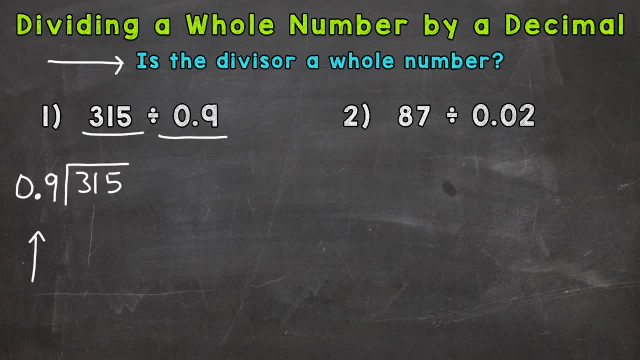 and for this particular problem, we need to push that 9- one spot or one place value to the left, so it's 9 ones or 9, and we can do that. Let's shift the decimal once to the right and therefore push that 9 over to the ones place. Okay, and this is the same thing. we are multiplying that 9 tenths. 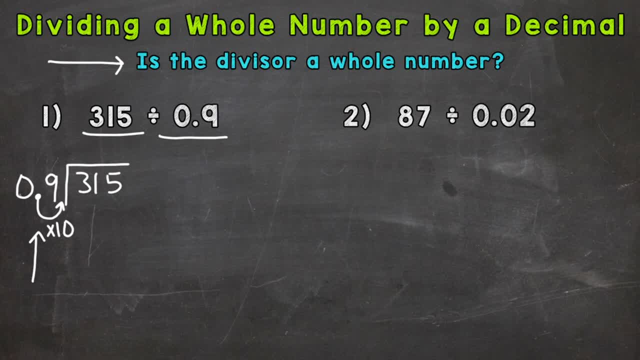 by 10 in order to divide that whole number by a decimal. So let's do that Now. you see that every time we multiply by a decimal, the decimal is being divided out, and we have to do that in order to get 9 whole. So we have a whole divisor now. but whatever we 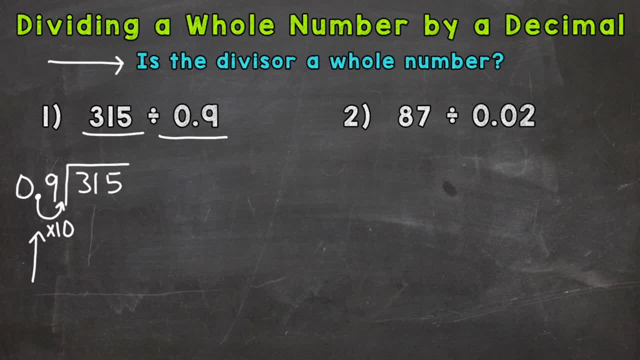 do to the outside, we have to do to the inside in order to keep this problem balanced and not change the value of the overall problem. So we need to multiply the inside number by 10 as well, So the decimal comes at the end of any whole number. so let's push each digit to the left once by moving the decimal once to the right. 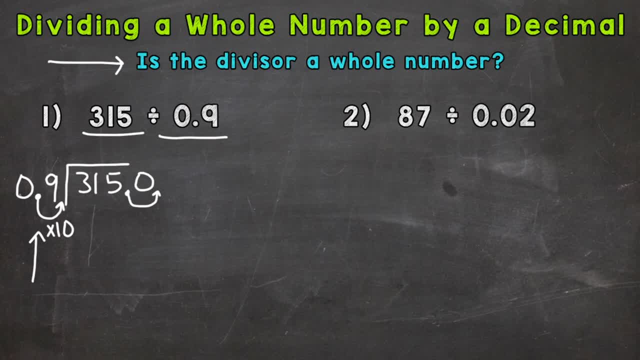 So now we can rewrite the problem without those arrows underneath and make it a little more neat and easier to work with. So we have 9 on the outside the divisor and we have 3,150 as our dividend, And the decimal is at the end here, the end of a whole number. So now we're ready to go. 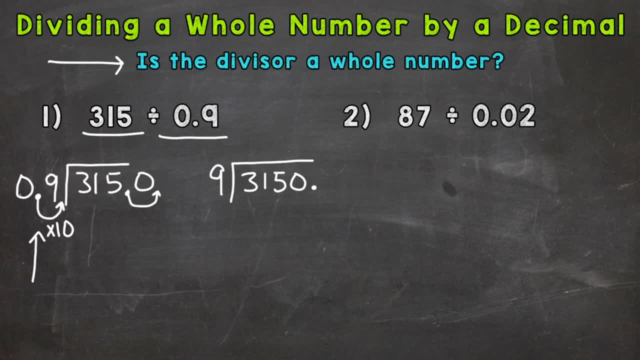 through the division process: Divide, multiply, subtract, bring down and repeat. So we have 3 divided by 9. And we can't pull any whole groups of 9 out of 3, so we need to use the 31.. So how? 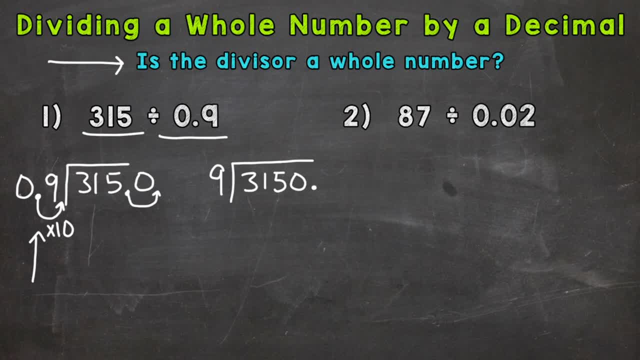 many whole groups of 9 out of 31?? Well, 3 nines gets us to 27, and that's as close as we can get. So 3 times 9, 27.. We subtract, Remember to borrow, We have to borrow here. So 11 minus 7 is 4,. 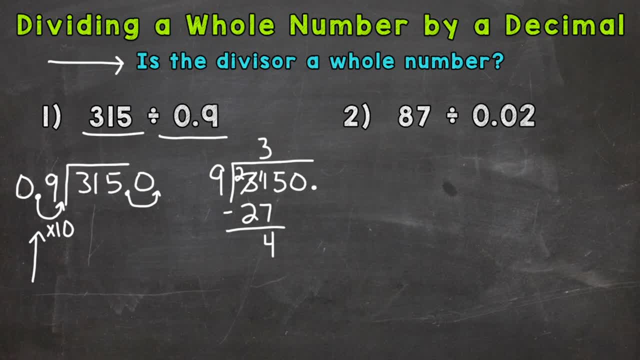 and 2 minus 2 is 0. So we get a difference of 4.. Now let's bring down our 5.. So now we have 45 divided by 9.. How many whole groups of 9 out of 45? Well, 5. 5 times 9 is 45. 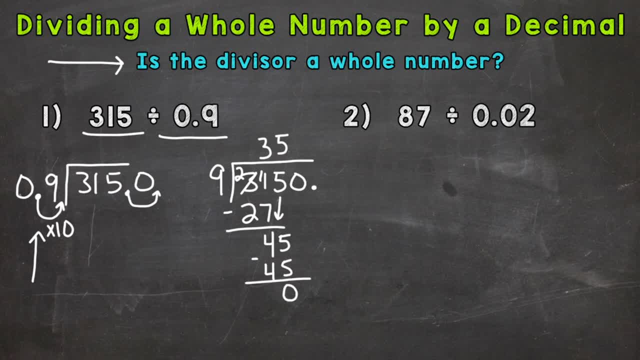 Subtract, We get 0. That 0 does not mean we are done with the problem. We need to go all the way over to the ones place and we still have a 0 to bring down. So we need something here. So we are. 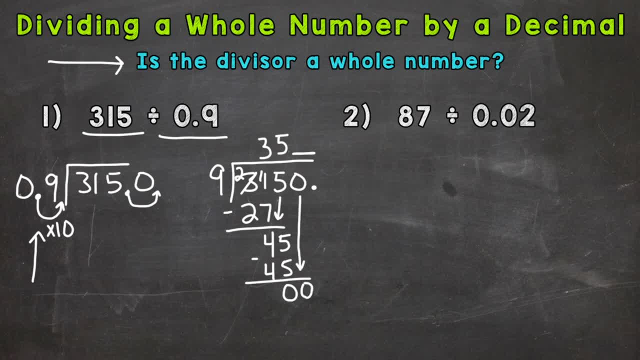 at the bring down step. And let's repeat: So: divide 0 divided by 9.. So how many whole groups of 9 out of 45?? Whole groups of 9 out of 0. Well, 0. We can't do that. So 0 times 9 is 0.. Subtract: We get a nice. 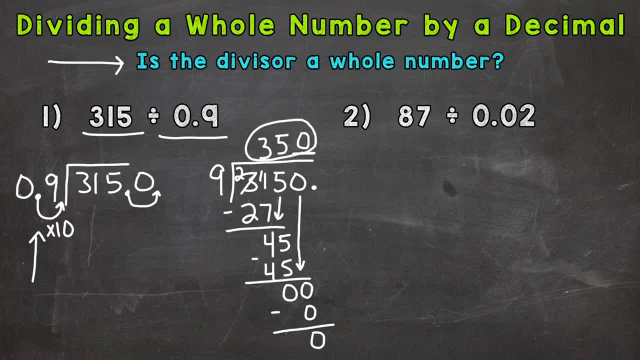 clean cut 0 there and an answer of 350.. So on to number 2, where we have 87 divided by 200.. Now this one's going to be a little bit different. Same process and everything, but you'll see what. 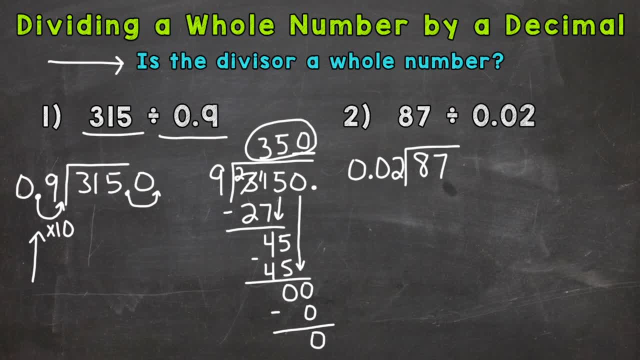 I mean here in a second. So the question we need to answer is how many whole groups of 9 out of 0? We need to ask ourselves: is the divisor a whole number? We have two hundredths, No, So we need to. 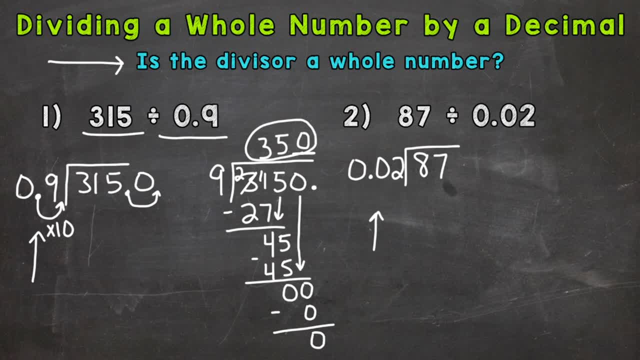 multiply by a power of 10 in order to make it a whole number. So let's see, If we shift each digit to the left once- and we can do that by shifting this decimal to the right- would we have a whole number? No, So we need to move it again. So we need to move the decimal twice here to get a whole 2. 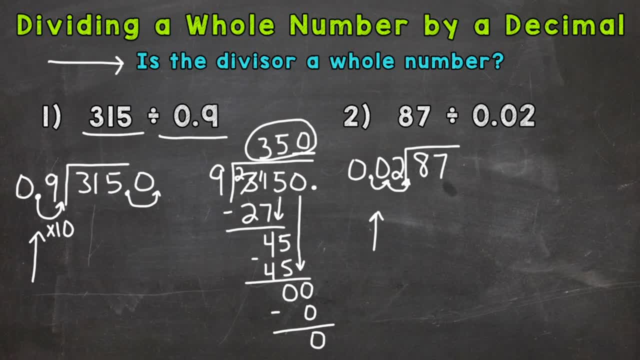 and push that two spots to the left to the ones place. So one time is times 10 times 10.. So we multiplied it by 100. 10 times 10.. So we need to multiply 87 by 100 or move the decimal twice to the right in order to push the 8 and 7 to the correct. 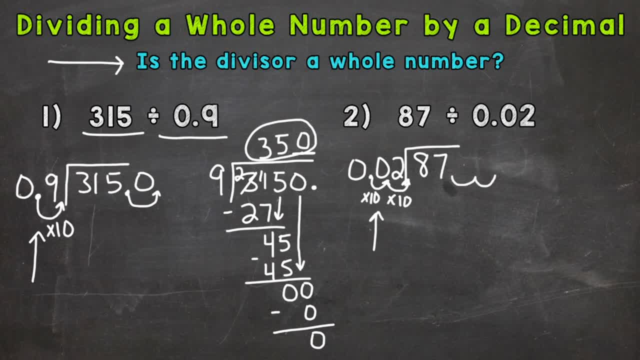 place values, So 1, 2.. Remember, the decimal comes at the end of a whole number. So I moved it twice to the right and we get 8,700.. So let's rewrite our problem with our whole divisor of 2.. And we have 8,700 here, decimals at the end of a whole number. And now that we have a 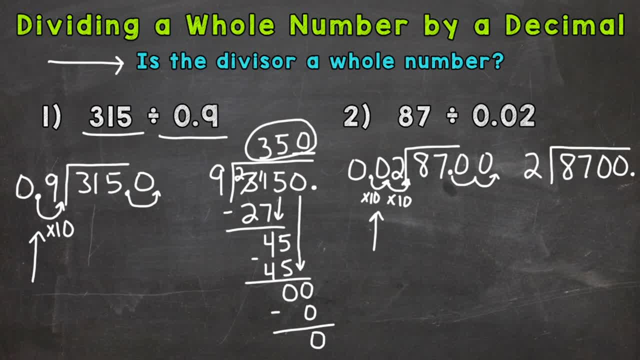 whole divisor. we are ready to go through our process. So 8 divided by 2 is 4.. 4 times 2 is 8.. Subtract we get 0.. Bring down the 7.. 7 divided by 2.. So how many whole groups of 2 out of 7? Well, 3.. That gets us to 6.. 3 times 2 is 6.. 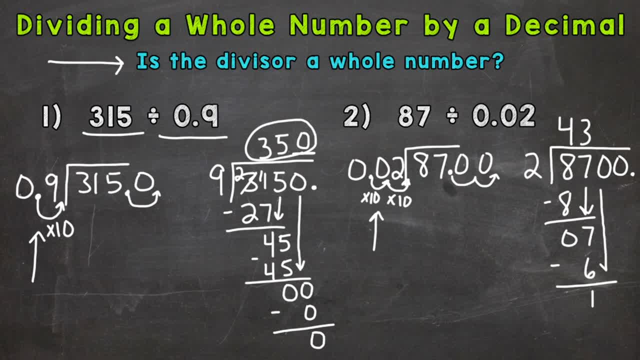 Subtract, We get 1.. Bring down the zero 10 divided by 2.. So how many whole groups of 2 out of 10? Five, 5 times 2 is 10.. Subtract: We get zero. But we are not done. We need to go all the. 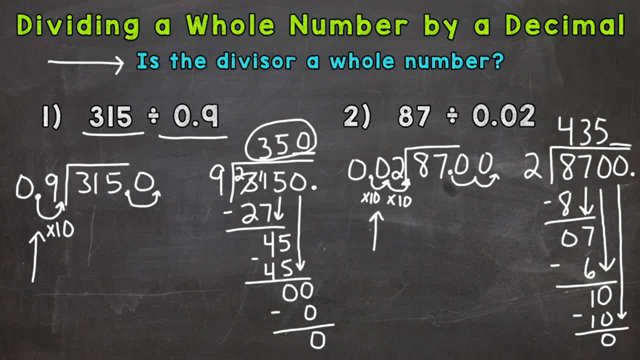 way over. So let's bring our 0 down. here We have 0 divided by 2.. So how many whole groups of 2 out of 0.. Well, 0.. We can't do that. So 0 there, 0 times 2 is 0 running out of 5.. I can't do that. 0 divided by 2 is 0.ared because of. time. 0 divided by 2.. So how many whole groups of 2 out of 0.? Well, we can't do that. So 0 divided by 2 is 0.. Running out of 5 is 0.. Running out of 5 is 3.. 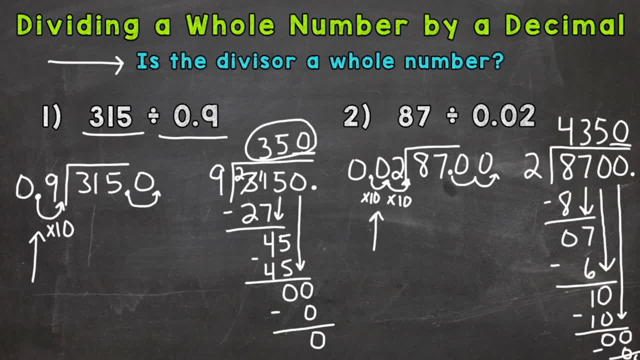 0 running out of room. 0 minus 0 is 0. squeeze it in that corner there. so we are all done. we get to a clean-cut: 0 and an answer of 4,000. I'll put a comma that is not a decimal: 4350. so there you have it. there's how you divide a whole number. 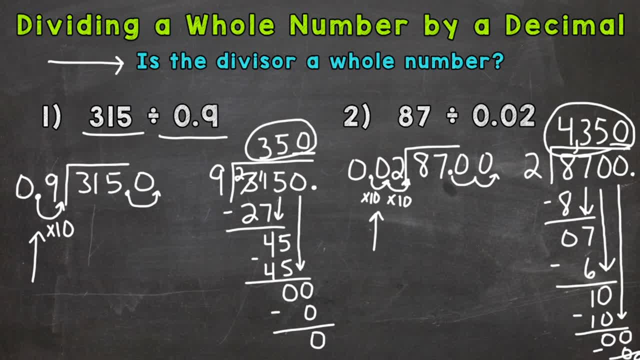 by a decimal. we always need to ask ourselves: is the divisor a whole number? when we see decimals within a division, problem. if it's not a whole number, we need to multiply it by a power of 10 in order to make it a whole number. whatever you do to the divisor, the outside number, you need to make sure you do to the. 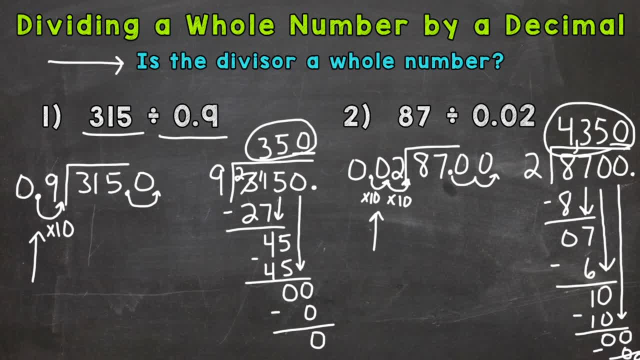 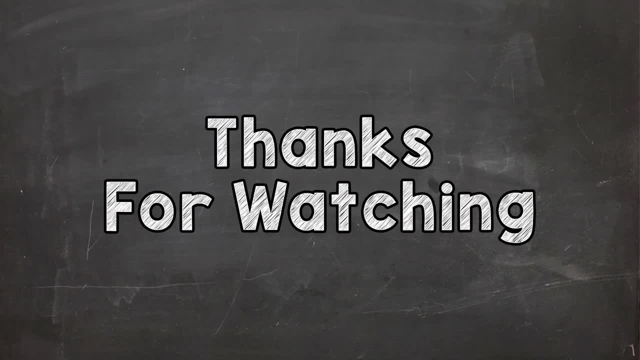 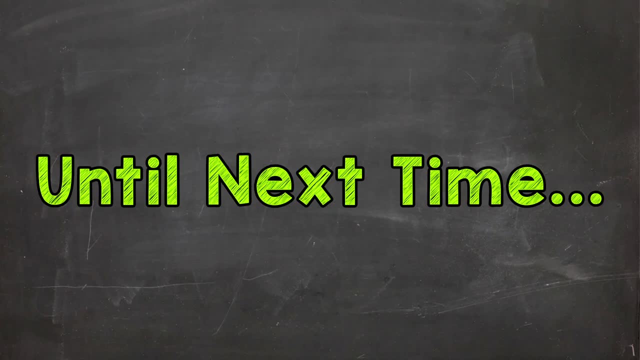 dividend the inside number and then go through your division process, and that will put you on the path to getting the correct answer. so I hope that helped. thanks so much for watching until next time, peace you.